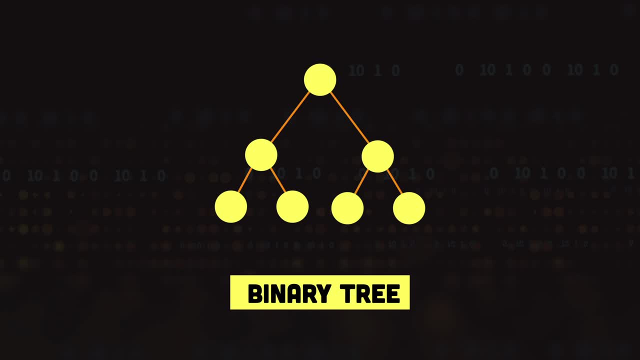 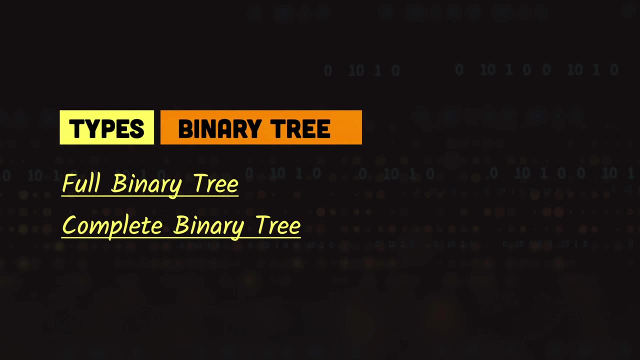 node of the tree could have maximum two children. There are different types of binary trees, but let's look at the full and complete binary trees before we talk about the heap data structure. All right, so full binary tree is the type of binary tree in which each node of the tree has 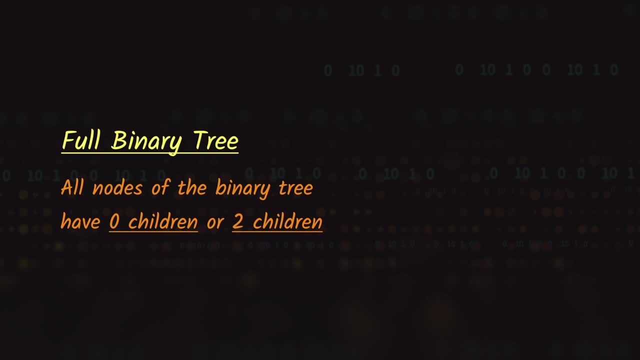 either no children or two children- Again no children or exactly two children. We can't have a node with one child. Let's take an example to understand this better. If you look at this tree, you can see that all the nodes of the tree have either two children or they are the leaf nodes. 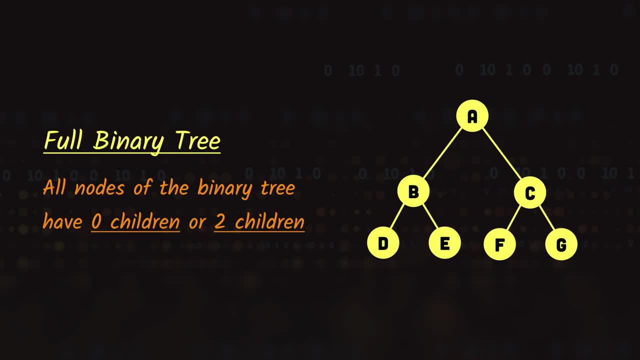 That is, they don't have any children. and because it follows the properties of a full binary tree, it is a full binary tree. So let's take an example to understand this better. So we can say that this tree is a full binary tree, Let's say that we remove the node G. 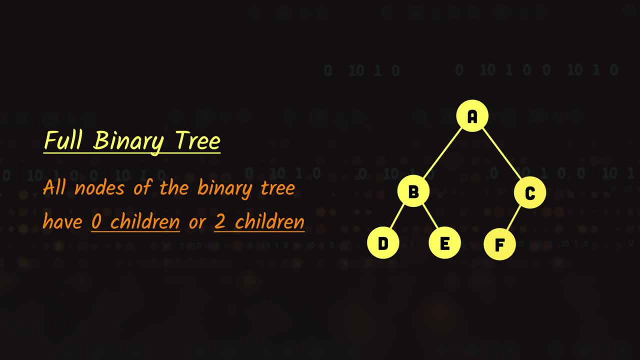 Now, in this case the tree will no longer be a full binary tree because the condition of full binary tree of having either zero children or two children is not being fulfilled because the node C has now one child. But if we remove the node F now it will become a full binary tree because C 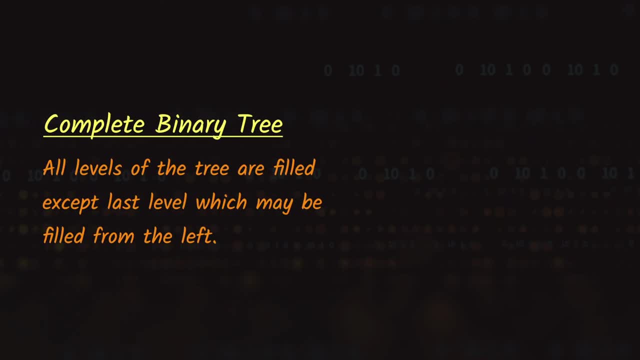 is a leaf now with zero children. Next we have the complete binary tree. In complete binary tree, all the levels of the tree are fully filled, except the last level, which can be partially filled. But the condition is that if we have any nodes on the last level, they must be. 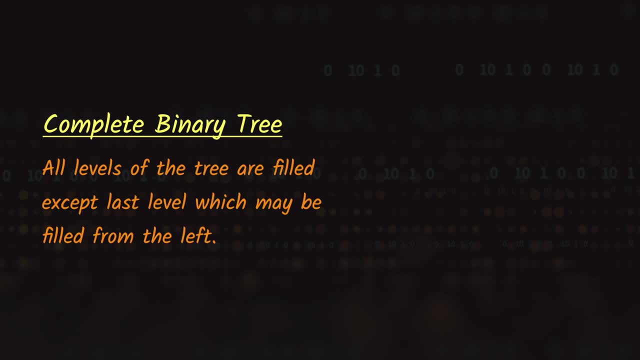 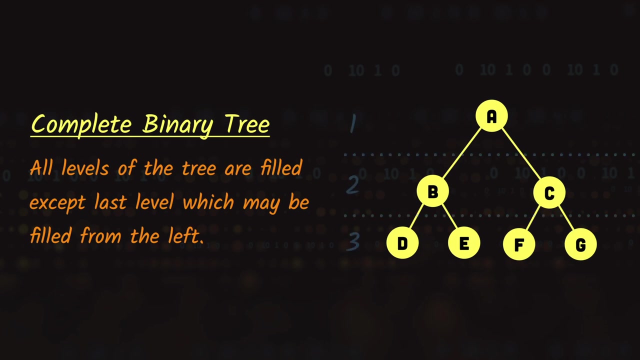 on the leftmost nodes. Again, all the tree levels are to be fully filled and the nodes on the last level should be on the far left side. Let's take an example to understand this better. So here we have a binary tree with three levels and you can see that all the levels 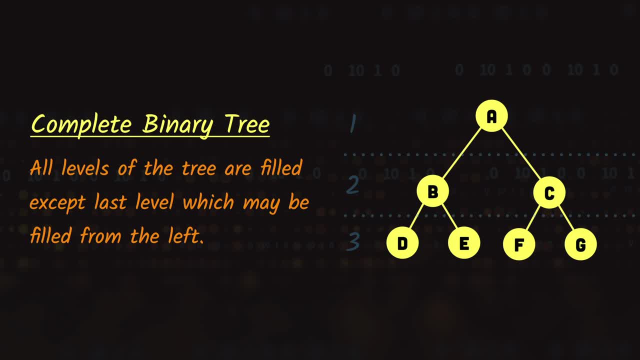 are fully filled with nodes, So we can say that this is a complete binary tree. Now let's say that we remove the node G. Now, if you look at the state of the tree, in this case, level 1 and 2 are fully filled and all the nodes on the level 3 are on the far left side. So it is. 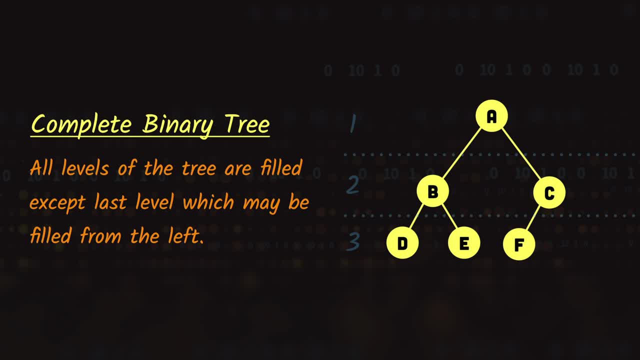 still a valid complete binary tree. Now let's say that we remove the node E. In this case, the tree is no longer a complete binary tree, since the condition for complete binary tree is to have all the nodes on the far left side, And node F in this case is not on the far left side. 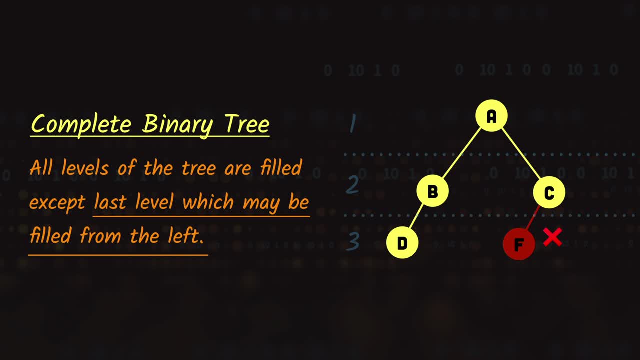 There are two ways to make this tree a complete binary tree. We can either move E under the node B or we can completely remove the node F. In both the cases, the tree will be a complete binary tree. Alright, enough about the trees, Let's look at the heap data structure. 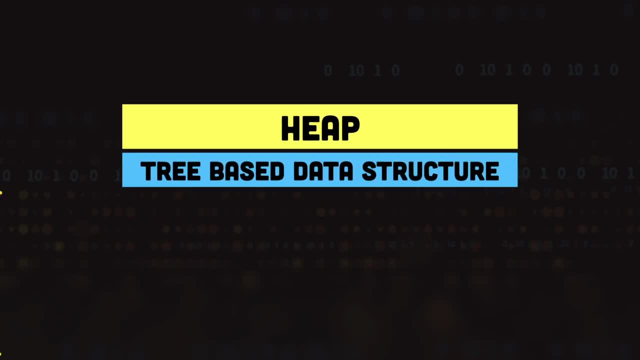 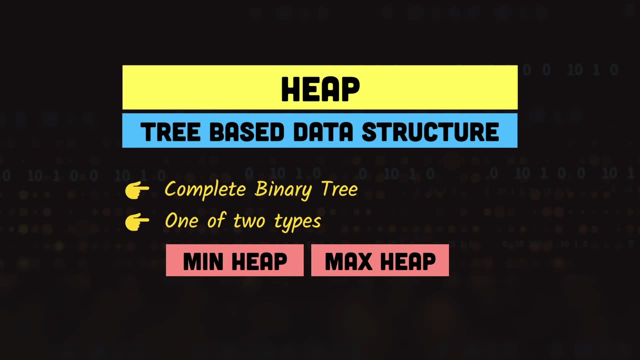 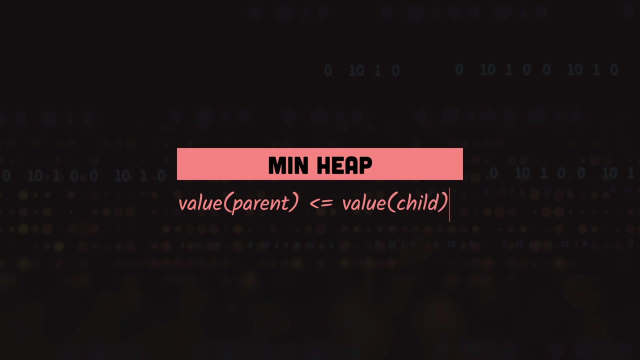 Heap data structure is the tree based data structure with two properties. First, it is a complete binary tree and the second it follows the properties of either min heap or max heap. Let's look at the min heap first. In min heap, the value of each of the parent. 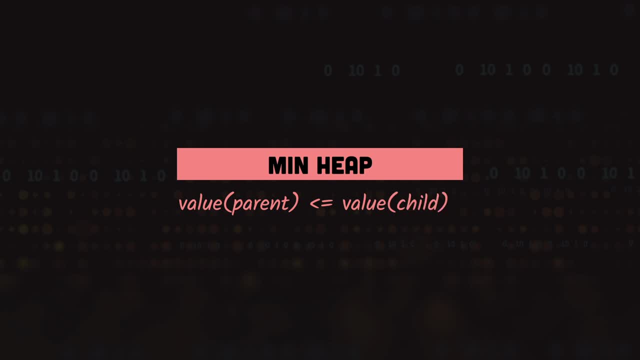 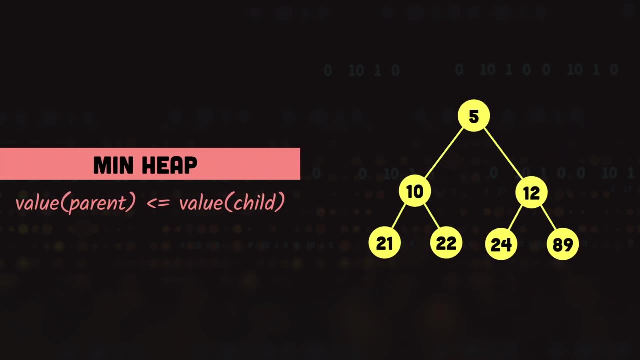 node of the tree is less than or equal to the value of its children. Let's look at an example to understand this better. Let's say that we have this binary tree with these values. Now, if you look at the node values, you can see that the value of each parent node in 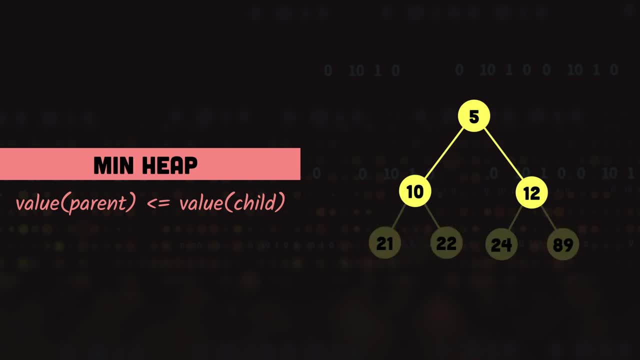 the tree is less than its children. So 5 is less than 10 and 12,, 10 is less than 21 and 22, and 12 is less than 24 and 89. And because the tree is fulfilling the properties of a heap and a min heap, we can say that the tree is a min heap. 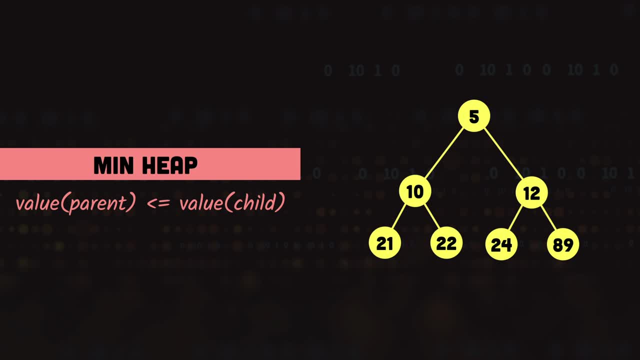 Now, before we go ahead, if you look closely at this min heap, you will notice two things. First, the value of the root node, which is 5, is the smallest value of the tree. Now, if we keep going down the tree, the values keep increasing. 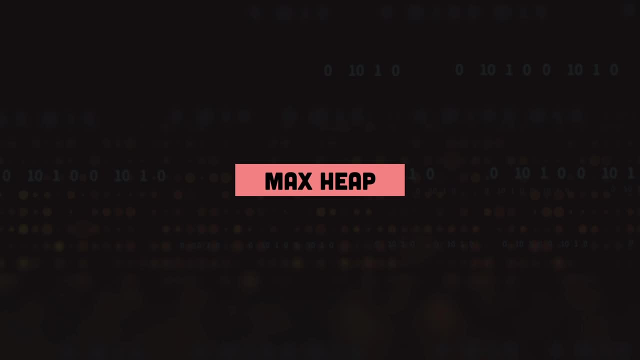 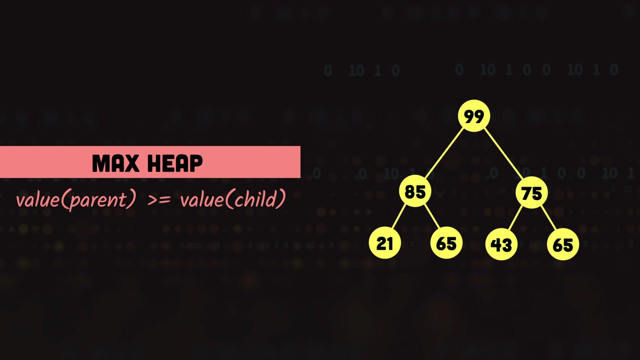 Alright. so next we have the max heap. Max heap is the opposite of min heap. That is the value of each parent node is greater than or equal to its children. Let's take an example. lets say that we have this binary tree with these values. If you look at the values here, 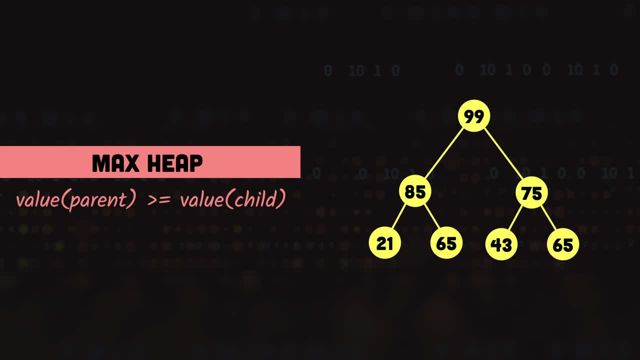 each parent node has a value greater than its children. So 96 is greater than its children. At least 99 degrees is greater than its children. 99 greater than 85 and 75.. 85 is greater than 21 and 65.. And 75 is greater than 43 and 65. 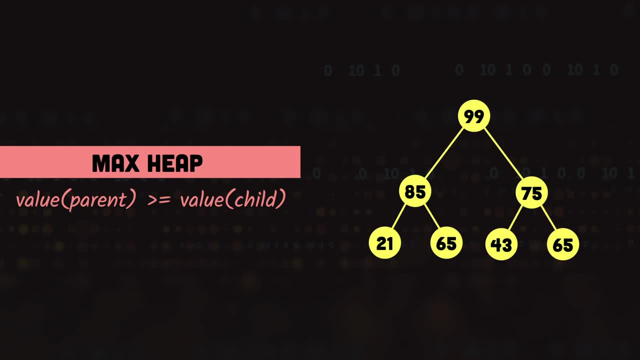 And because all the properties of heap and max heap are being fulfilled, we can say that this is a max heap. And also you can see that the value of the root node in a max heap is the largest value of the tree And also, if we keep going down in the tree, the values 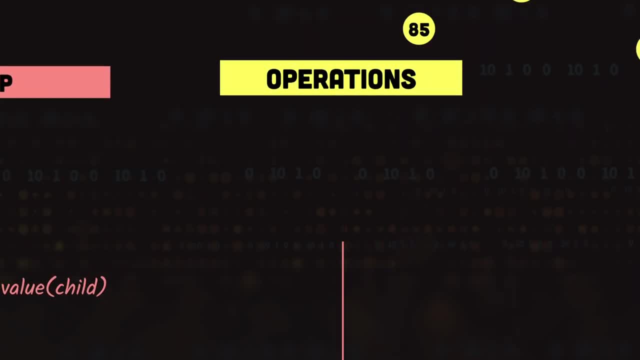 keep getting smaller and smaller. Alright, let's look at the heap operations. First of all, we have the insert operation. Insertions in heap are done from the top to bottom and left to right. Let's see how it works. Let's start with node 40, which will become the 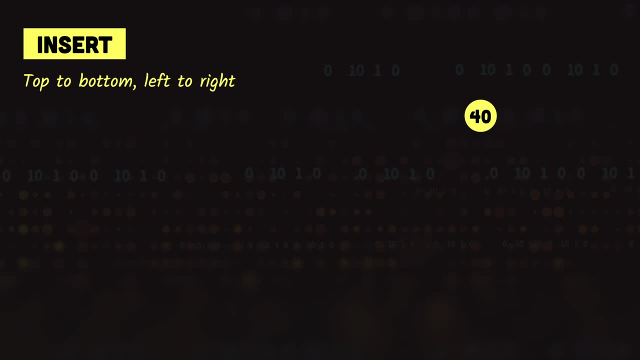 root node, because this is the first node of the tree. The next item, 31,, will be inserted to the left of the root node 34 will be inserted to the right of the root. node 98 will be inserted to the left of 31.. 9 to the right. 33 to the left of 34.. 11 to the 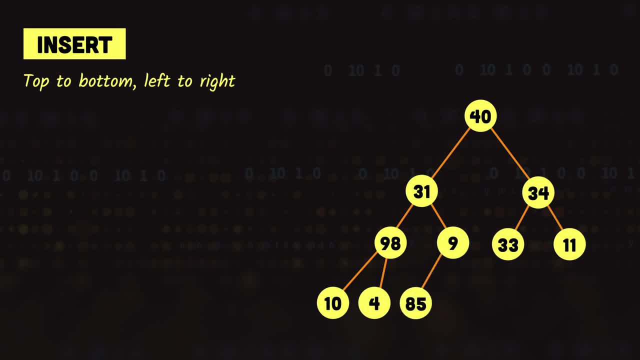 right of 34.. And similarly, we'll keep on inserting the new nodes from left to right. Alright, now, if we look at our tree, we have a problem here. It is not a heap, Because, as per the properties of a heap, it should be a valid, complete binary tree, which it is, But it 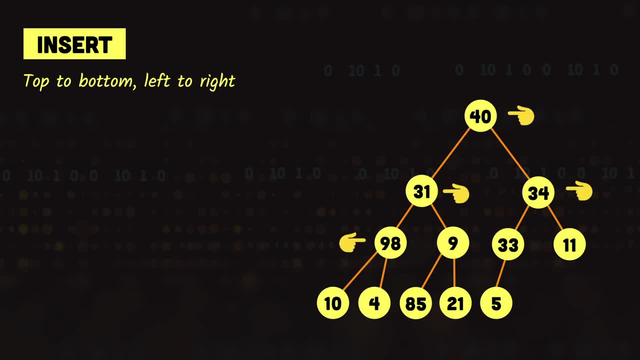 is neither a min heap, Because some parent nodes have a greater value than the children, And nor it is a max heap, Because some nodes have a smaller value than the children nodes. Alright, so how do we fix this issue? To fix this issue, after each insertion we compare the newly inserted. 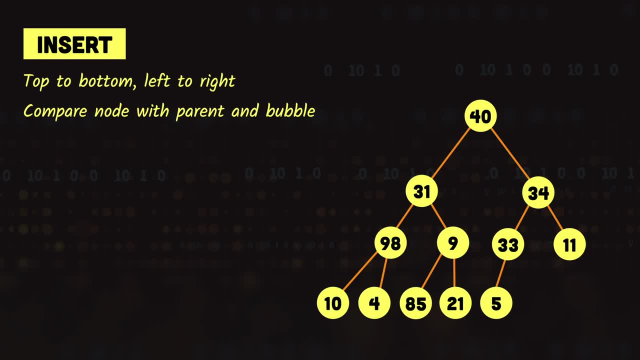 nodes value with the parent node And we bubble the node up if needed. Let's see how this bubbling works in a min heap. Let's say that we have 40 at first, Because this is the first node of the tree. Now we just add parts of the rural node, each new node. 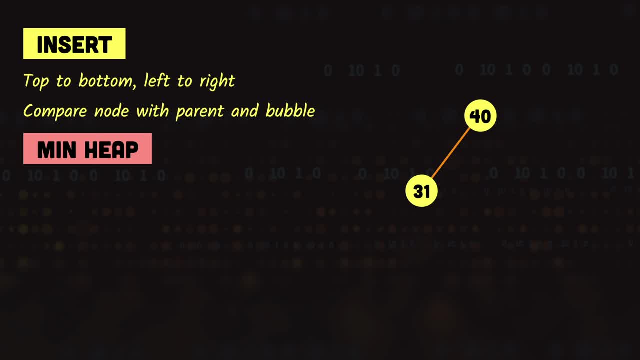 Next we have 31.. We'll insert 31 at the left of node 40. And after insertion we will compare the new node's value, which is 31,, with the parent node, which is 40. In the min heap the parent node must be smaller than the child node, So we'll simply swap. 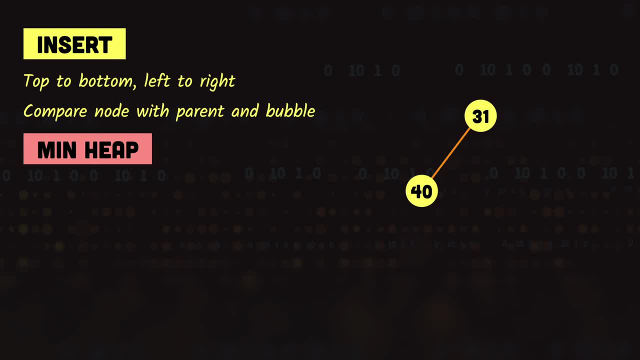 31 with the 40., And 31 will become the new root. So here we have a single parent node. Next we have 34. Which will be inserted to the right of the 31. The child: Now again, we will do the comparison. now, 34 is greater than 31, so no swap or bubbling. 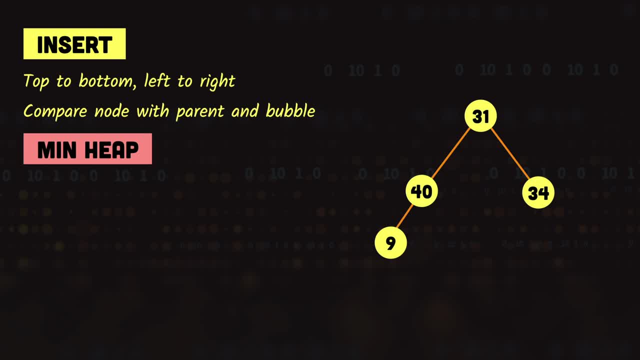 is needed. Next we add 9, which will be inserted to the left of 40. Again, we will do the comparison. 9 is smaller than 40, so 9 will bubble up. Next we will compare 9 with 31, and again 9 is smaller, so it will bubble up and become: 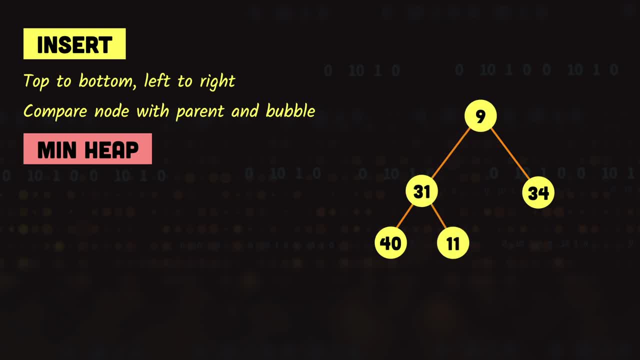 the new root node. Next we have 11, comparing 11 with 31,. 11 will move up. Comparing 11 with 9,: 9 is smaller, so no more bubbling is needed. Next we have 85,. 85 is already greater than 34, so no bubbling is needed. 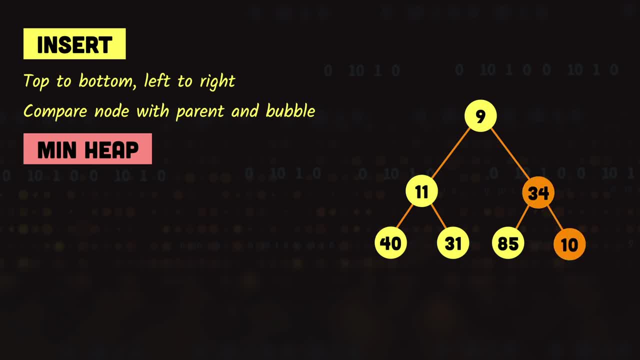 Next we have 10, we will compare it with 34, so 10 is smaller than 34, so we will bubble it up. After that, we have 10 and 9, 10 is greater than 9, so we will stop here and no more bubbling. 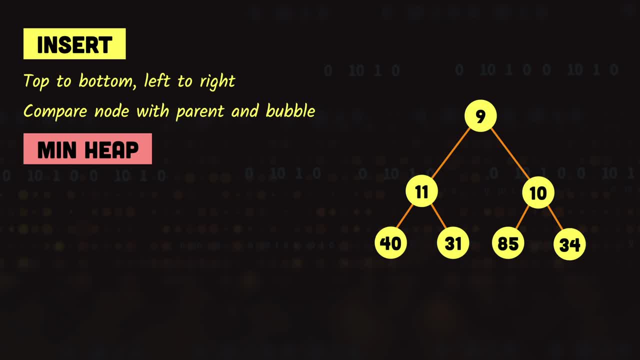 And this is how the new nodes are inserted. into a min heap, We insert the node and keep bubbling it up if the value of the node is smaller than the parent node. In the similar way, we have the max heap, where we insert a node and keep comparing and bubbling. 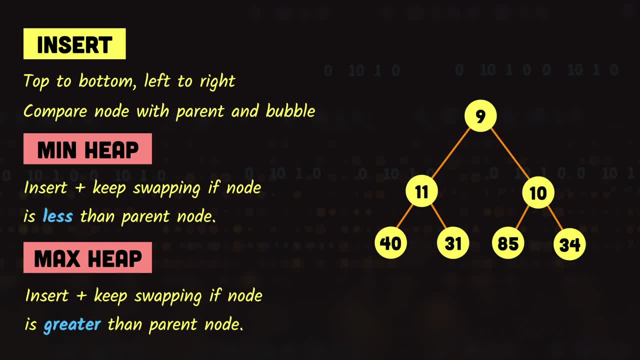 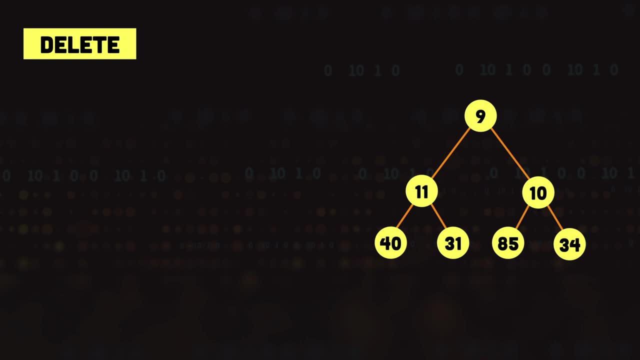 it up if the newly inserted node's value is greater than the parent node. The complexity of insertion in a heap, whether it is a min heap or a max heap, is logarithmic. Alright, so next operation we have is the deletion operation. While deleting a value from a heap, if it is a min heap, we delete the smallest value. 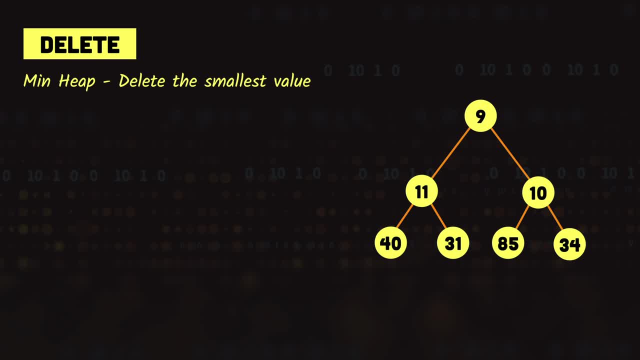 first, after that we delete the second smallest value, after that we delete the third smallest value, and so on. And similarly in the max heap we start with the deletion of the largest value and after that we delete the second largest value and then the third largest value, and so on. 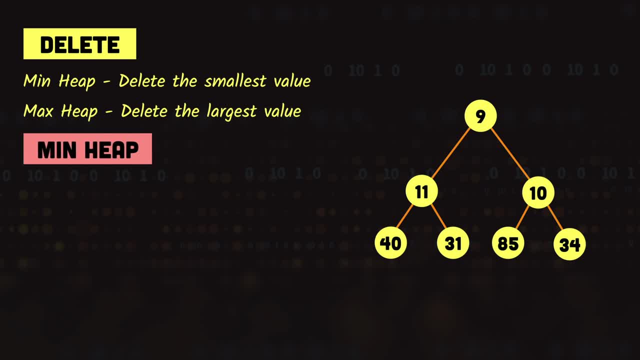 Let's see how we can delete items from a min heap 1.. The smallest value in the min heap is owned by the root node, So we will simply delete the root node. but now we have an empty space for the root. To fill this space, we pick up the last element of the heap and make it the new root. 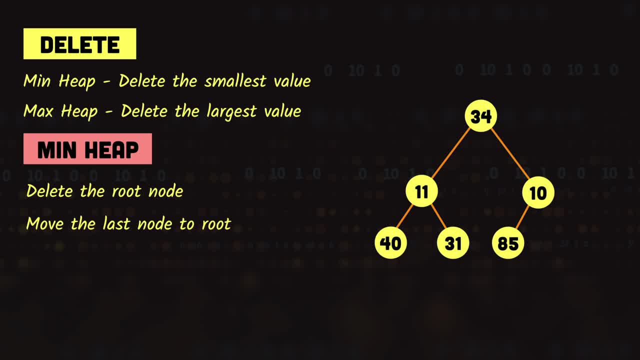 But the issue with this approach is that the new root that we may pick it may not be the valid root. So if you look at the current example, we have the root node of 34.. 34 is greater than the children nodes 10 and 11.. 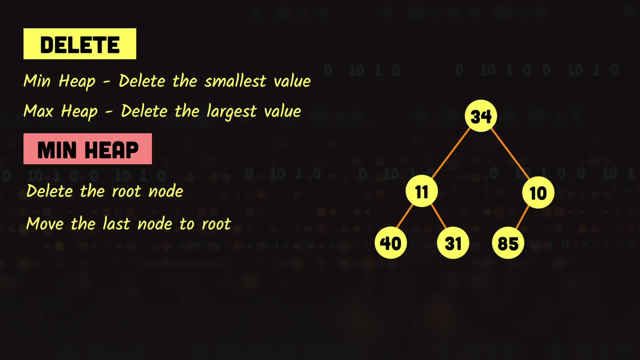 So our tree is not a min heap anymore. To fix this issue, we compare the new root with its children and bubble the node down till it reaches the place where it has to be. So in this example, we will compare 34 with 11 and 10.. 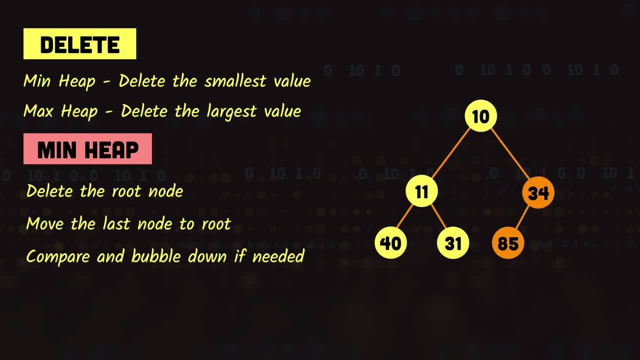 Now 10 is the smallest of the three values, so we will move or swap 34 with 10.. Next we will compare 34 with 85. Now 34 is smaller, so no more bubbling is needed. So this is how the deletion works in heap. 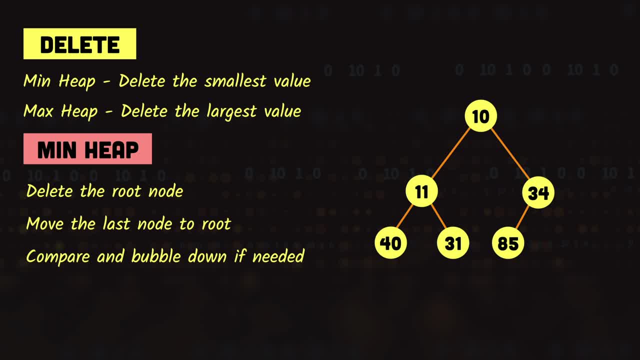 We delete the root node, Move the last node to the root position and bubble the root down till it reaches its position. Lets take another example to make sure that we understand this better. Next, we will remove 10 and we will move 85 to the root node. 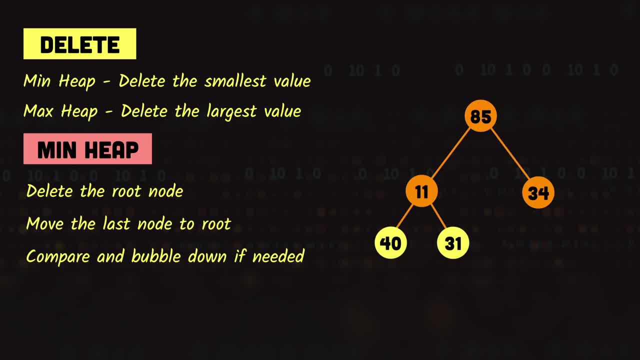 Now 85 will be compared with 11 and 34.. 11 is the smallest, so 11 will be swapped with 85.. Now 85 will be compared with 40 and 31.. 31 is the smallest. Its swapped with 31 and with that our heap will be ready after the deletion. 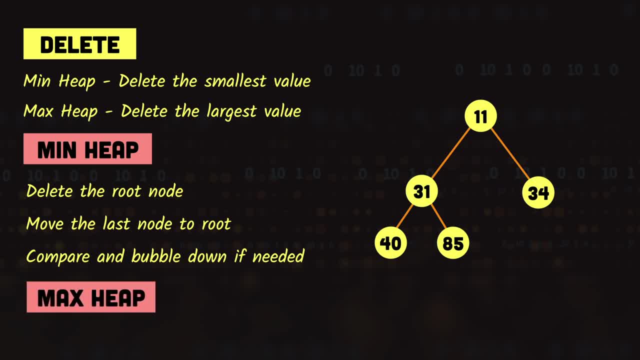 The deletion in maxheaps also works the same way. The only difference is that instead of looking for a smaller node value, we look for a greater node value when we bubble down the root node. The algorithmic complexity of deleting a value from a heap is also logarithmic. 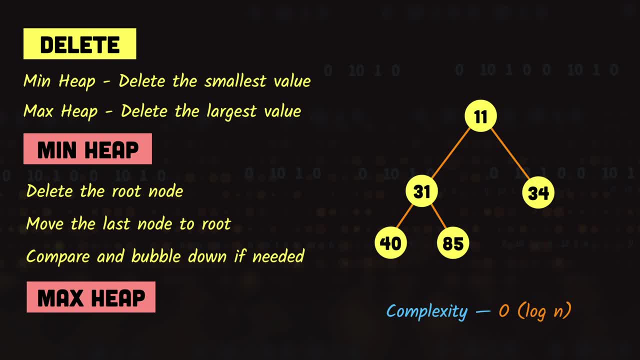 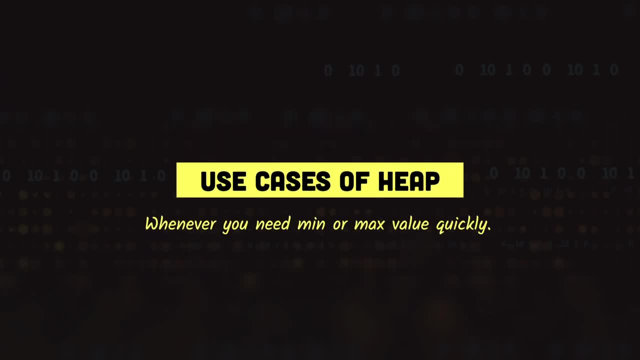 Alright. so now that we have covered what the heap is, the types of heap and the different heap operations, Lets look at the use cases of the heap data structure. The heap data structure is mostly used in the cases when we need to access the minimum. 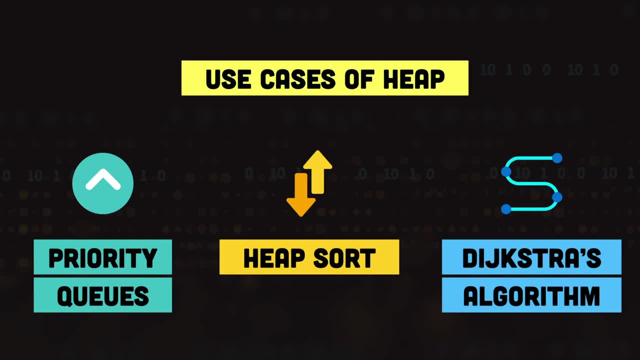 or maximum values quickly. They are used in the priority queues. for example, if you have a list of tasks with importance assigned to each task And while working on a task you move from the highest importance task to the lowest importance task, In that case you might want to use priority queue or a heap.